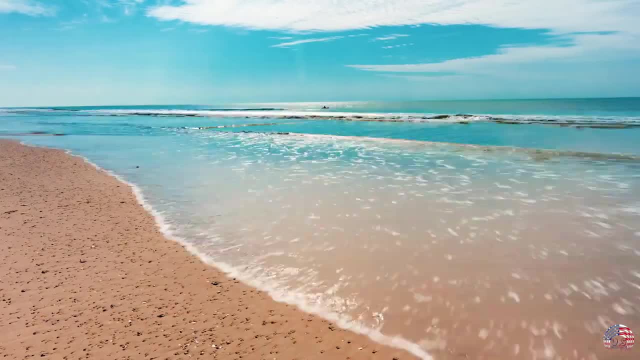 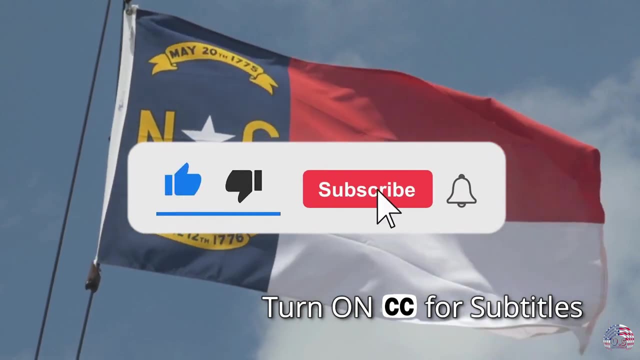 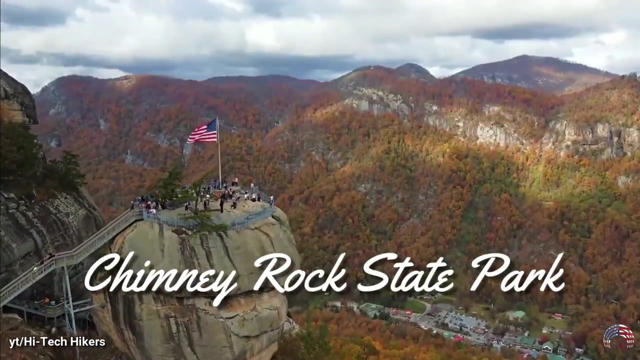 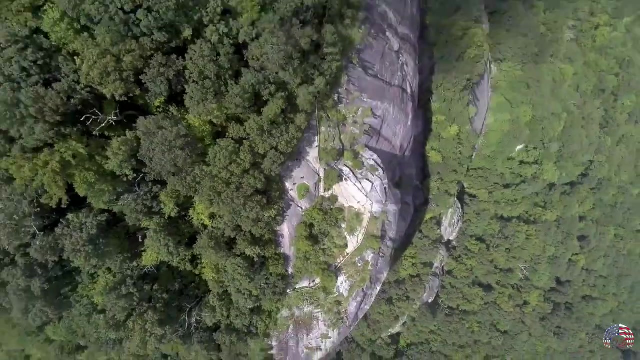 Here's a list of the top destinations to visit within North Carolina, So you will be notified for our next videos. The park is situated approximately 25 miles southeast of Asheville and offers miles of trails for hiking and the stunning 400-foot Hickory Nut Falls. 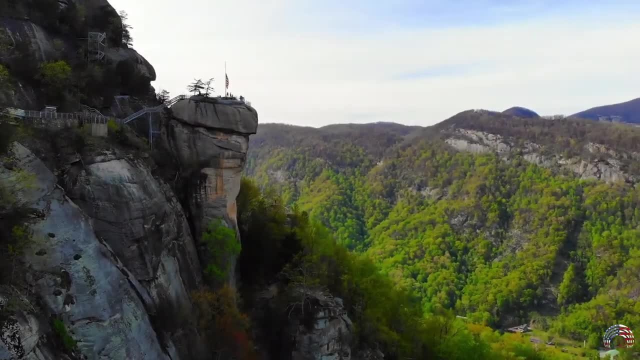 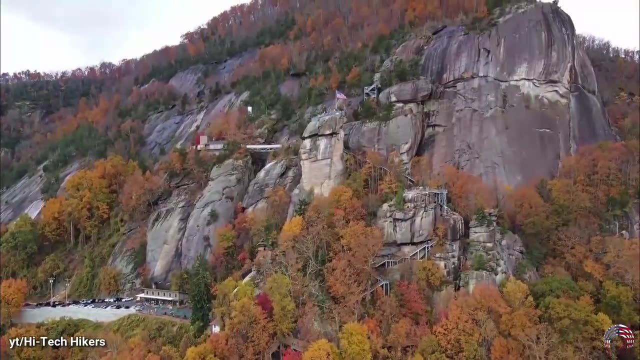 The most renowned attraction in this national park is over a 300-foot monolith, also known as the Chimney Rock, offering stunning views of the surrounding area. The 300-foot monolith is the most famous attraction in North Carolina. The 815-foot granite spire rises to over 2,280 feet in Chimney Rock State Park. 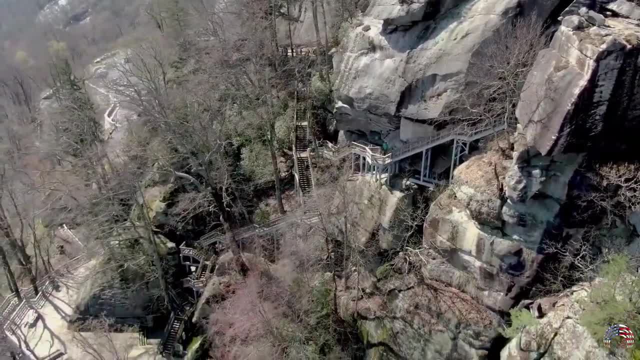 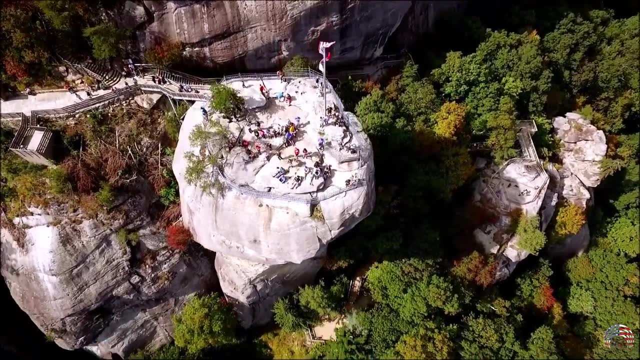 Don't be worried about the pressure and stress in climbing the mountain, as there's an elevator with 26 stories Built into the mountain, making an easy journey for visitors, where you can climb the 500 steps at the very top of the chimney. 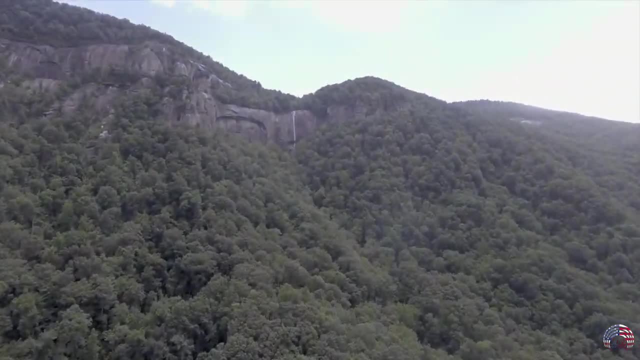 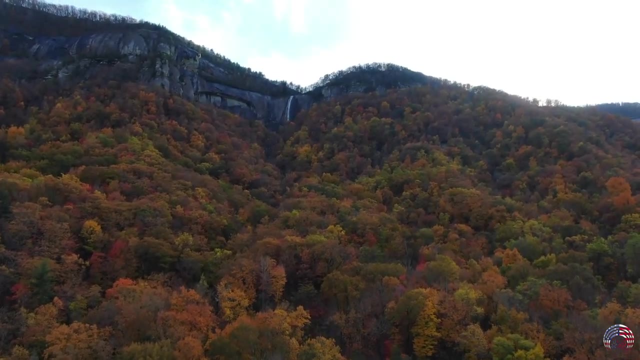 In the park you can hike the Hickory Nut Falls Trail, mostly an easy trail, leading to Hickory Nut Falls Base. The stunning waterfall tumbles off the sheer red rock- The park is also known as Flat Ledge- before disappearing into the surrounding trees. 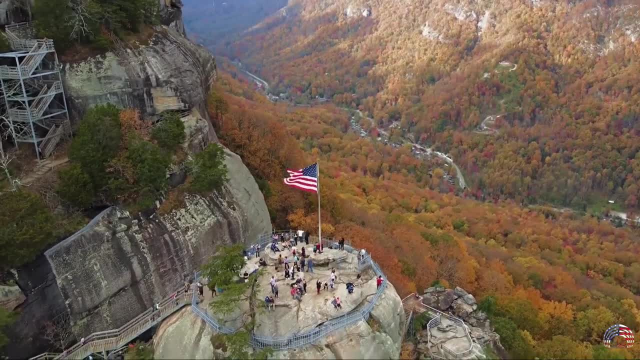 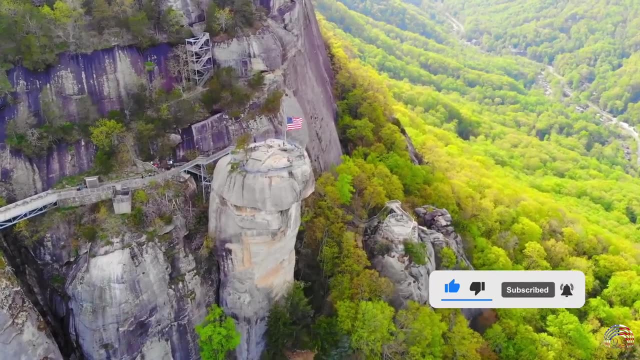 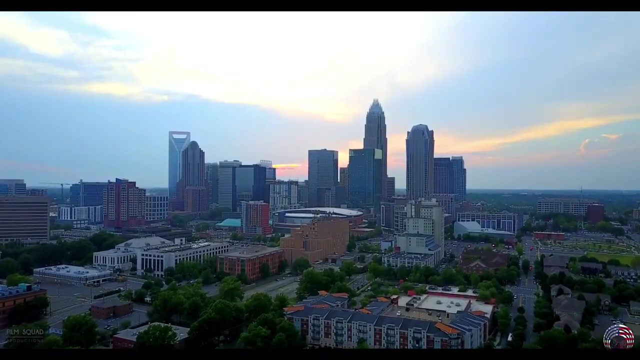 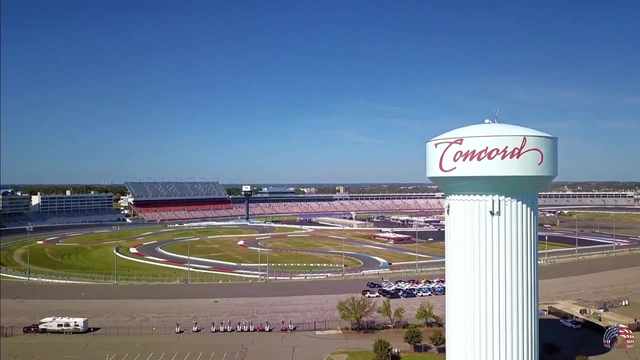 The park is relatively new and was only granted permission through the North Carolina General Assembly in 2005.. Charlotte: It's a major city and commercial center of North Carolina. Charlotte is the biggest town and offers many things to provide visitors, particularly those who enjoy motorsports. 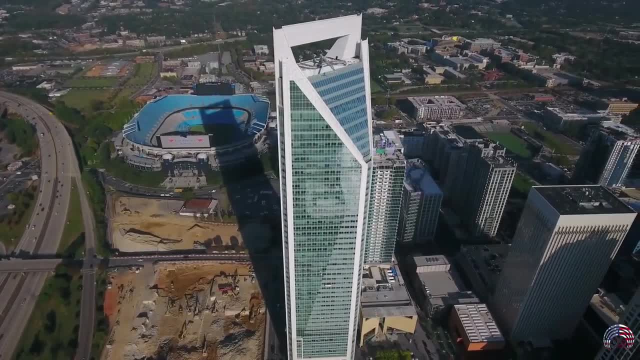 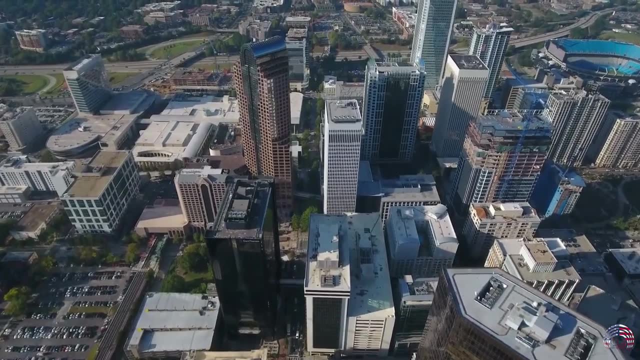 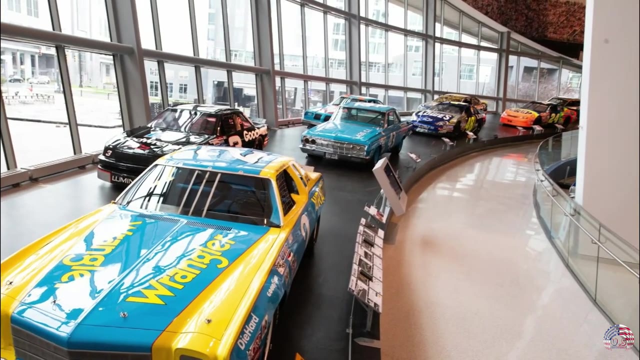 The Levine Museum of the New South is located in Uptown. The city's modern center explores post-Civil War history and has hands-on science exhibits at Discovery Place. The NASCAR Hall of Fame is another landmark in Uptown and it celebrates auto racing with interactive exhibits and films. 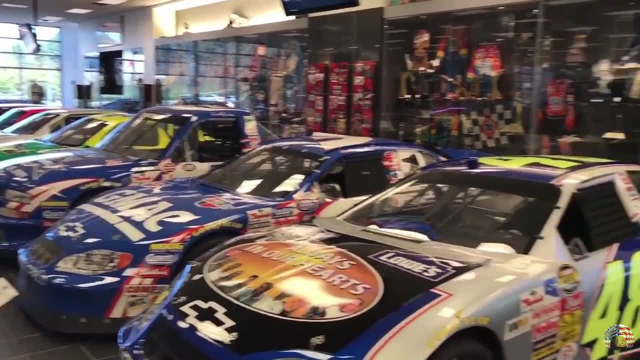 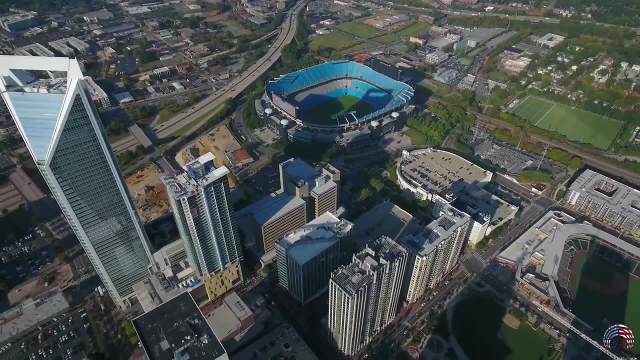 Additionally, nearly every NASCAR racing shop is open to all visitors in the suburbs around Mooresville. It is known as Queen City, home of various exciting attractions like the Carowinds Amusement Park, and is the home of some of the world's largest art-famous connaissance parks. 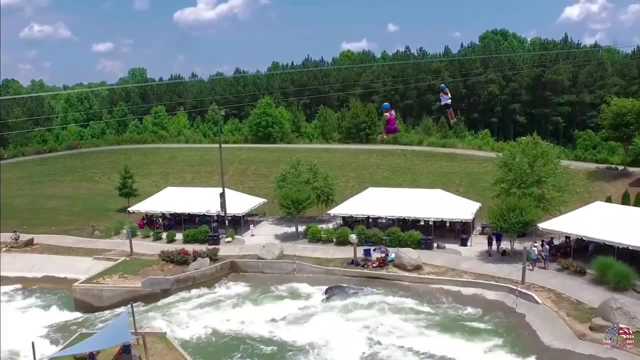 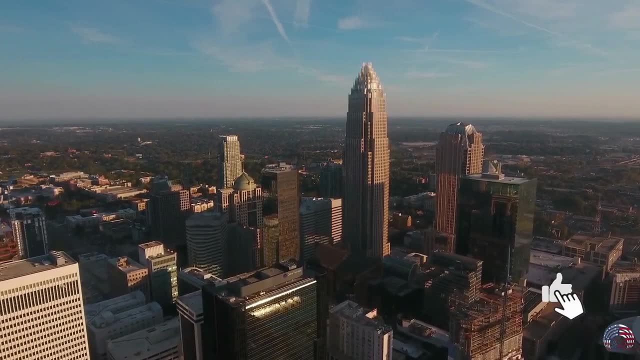 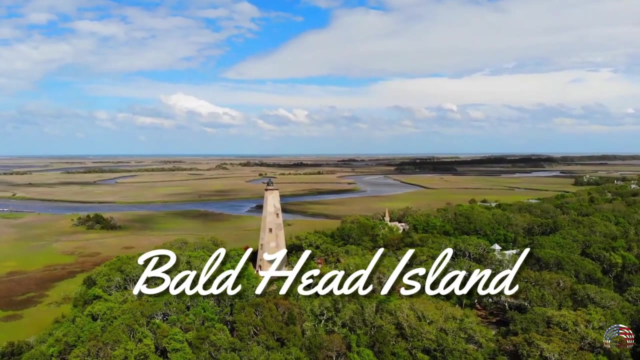 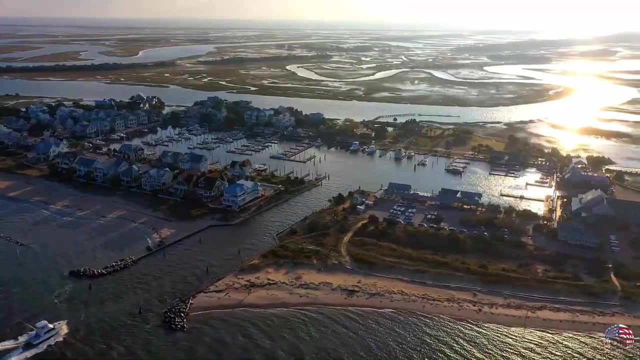 The Whitewater Center is a family-friendly venue to explore the beautiful Baltimore. The Whitewater Center is the world's largest artificial whitewater park. The US National Whitewater Center is a family-friendly place with a science museum and an aquarium. a ferry from Southport. The town of Southport has 14 miles of sandy beaches and a peaceful atmosphere. The best way to travel is on bicycles or golf carts. The island's landscapes have marshes, maritime forests and baldhead golf course. It is also a nesting site for turtle. 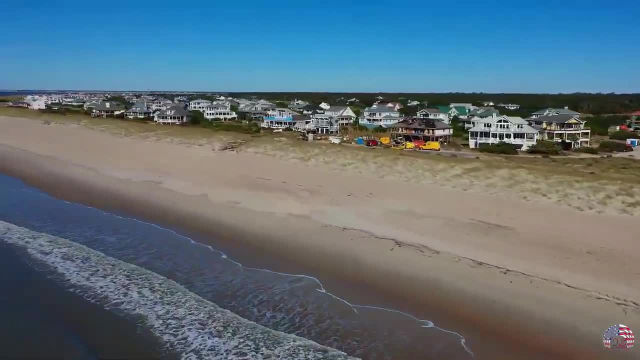 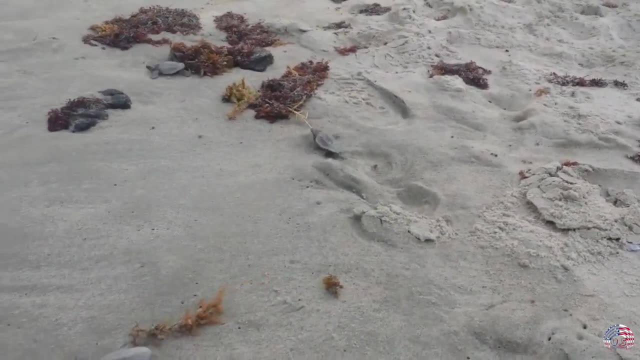 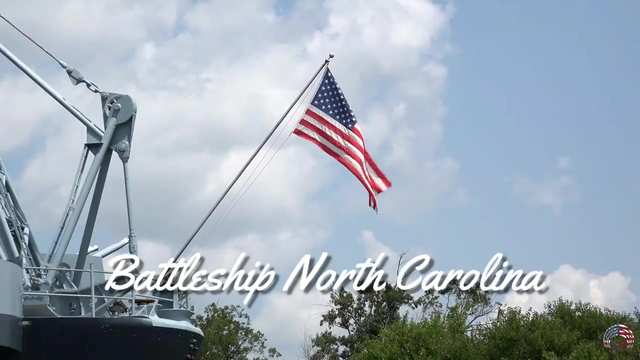 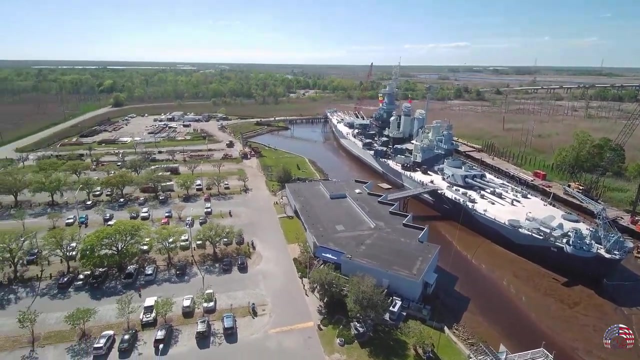 during the summer months, The Baldhead Island Conservancy hosts turtle walks for visitors who would like to see the nest of turtle babies or turtles arriving on the beach to build a nest. 3. Battleship North Carolina. The ship is located in Wilmington, the USS North Carolina was the first of 10 battleships. 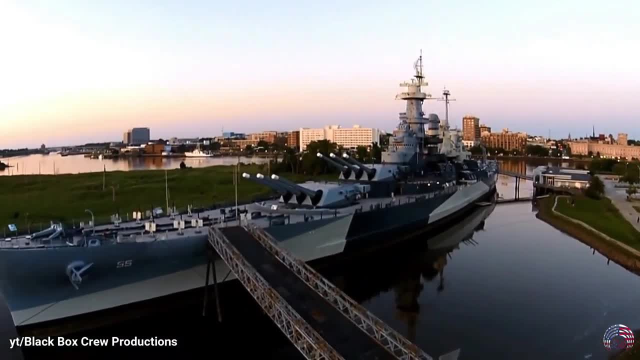 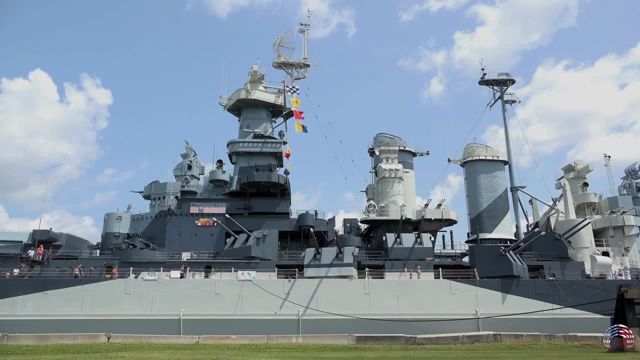 that would become part of the American fleet during World War II, after being launched on April 9, 1941. The ship was equipped with 9 16-inches rifles, 3 45-caliber turrets, 25-inch guns of war and a 7.5-inch gun. The battleship was also equipped with a. 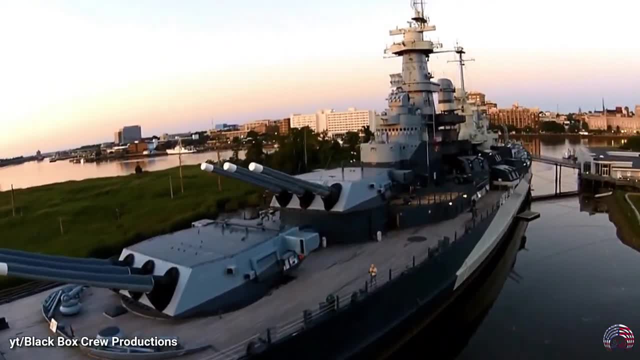 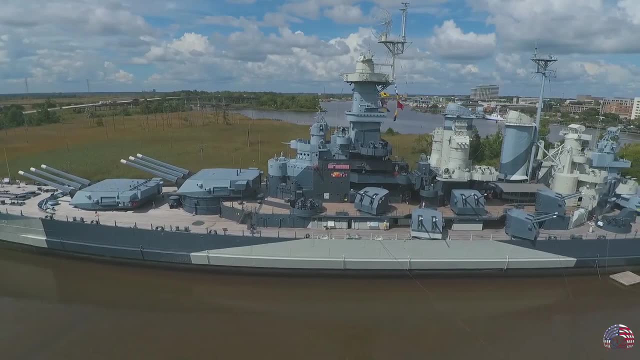 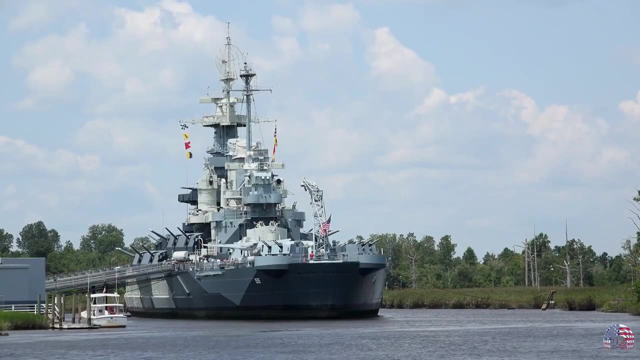 38-caliber and 10 twin mounts. All of these weapons are still functional today, but visitors can only see them. It was once the world's most powerful sea weapon, but today her guns are secluded. To appreciate this vessel's immense force, explore the vast deck and see the 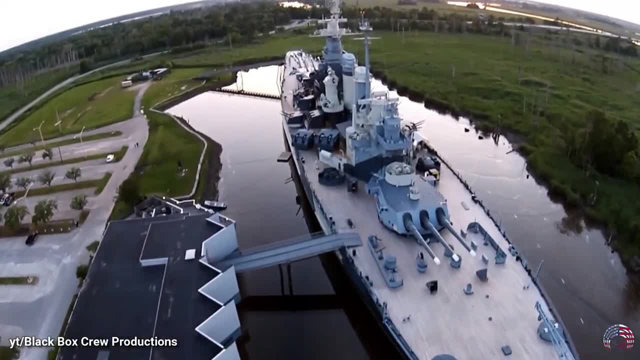 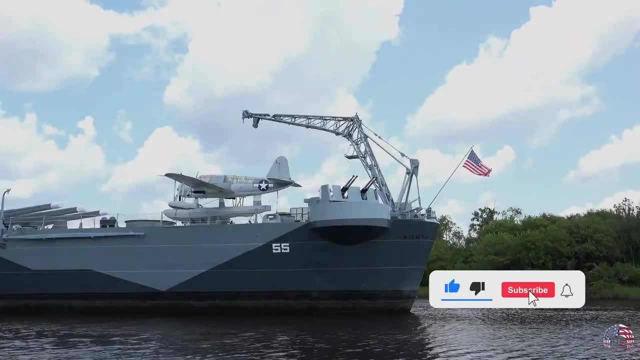 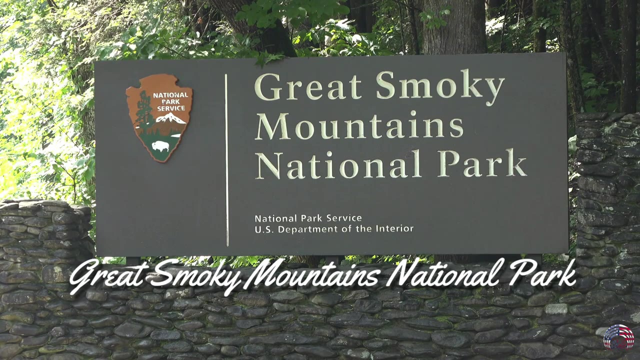 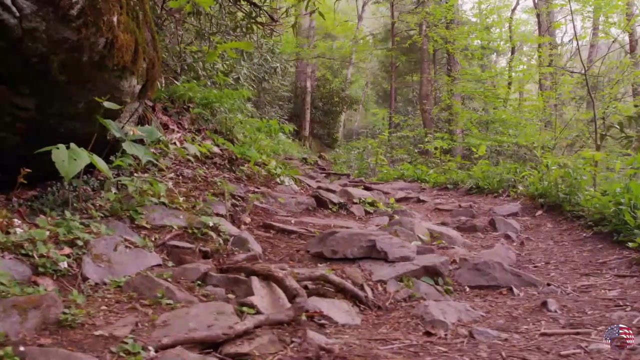 impressive guns in close proximity. The ship's other areas are also accessible. be sure to check out the mess hall and visit the officers' and sailors' quarters. 4. Great Smoky Mountains National Park. Located on the border of North Carolina and Tennessee, This sprawling area is home to 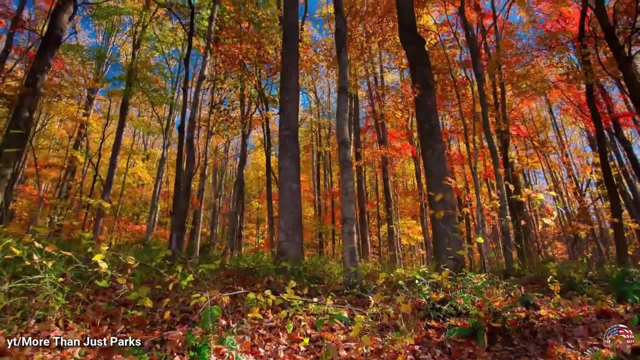 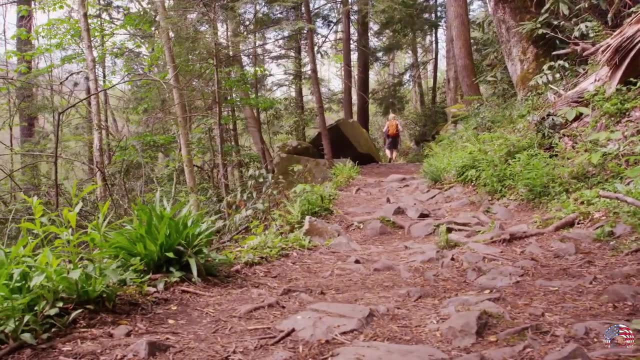 lush forests and a wide variety of wildflowers in full bloom. There are several streams, rivers and waterfalls, along with hiking trails that connect to the Appalachian Trail. Clingman's Dome is the highest peak and offers breathtaking views of the most covered mountains. 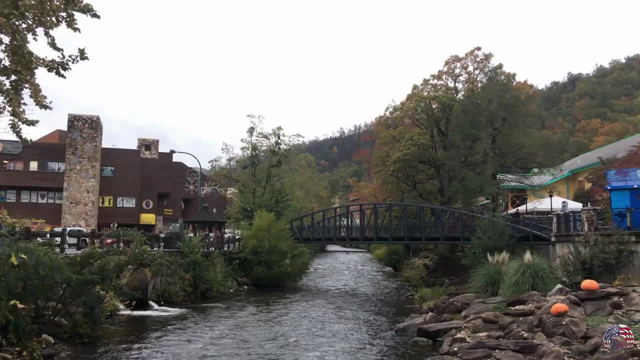 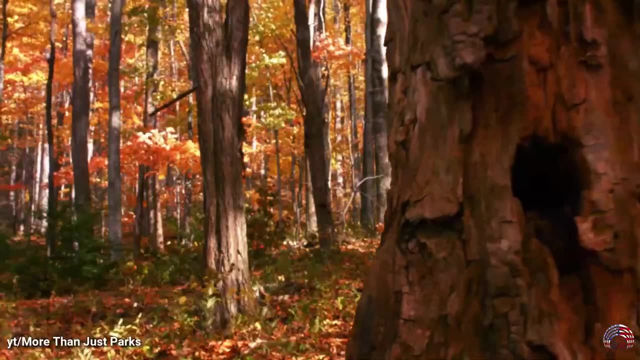 from an observation point. Clingman's Dome is the highest peak and offers breathtaking views of the tower. The park is in easy reach from several major East Coast cities and it is the most frequented national park within the United States. The accessible nature makes the park famous. 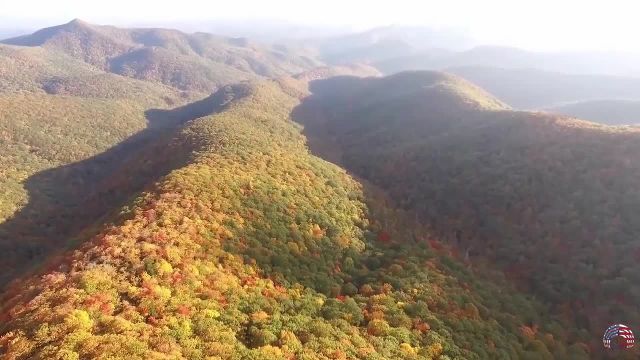 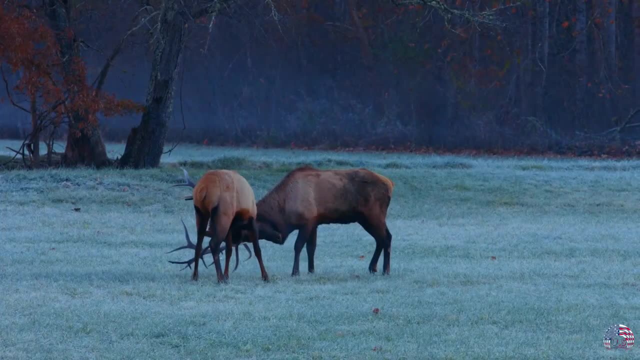 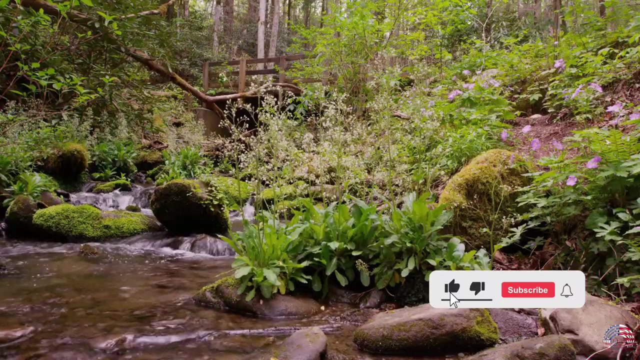 also known for its abundance of wildlife and breathtaking landscape. It's home to more than 1,500 black bears, along with deers. foxes, turkeys and even elks were recently brought back to the park. Furthermore, the park has 885 miles of trails and numerous beautiful 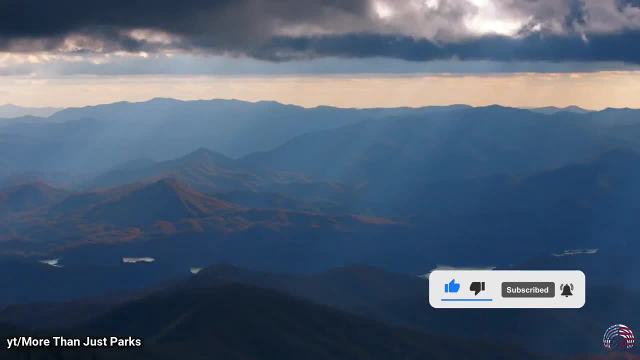 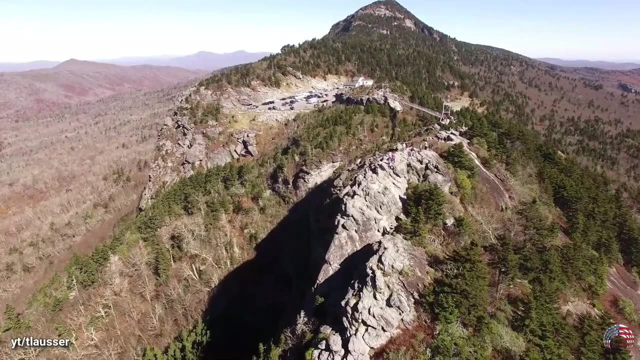 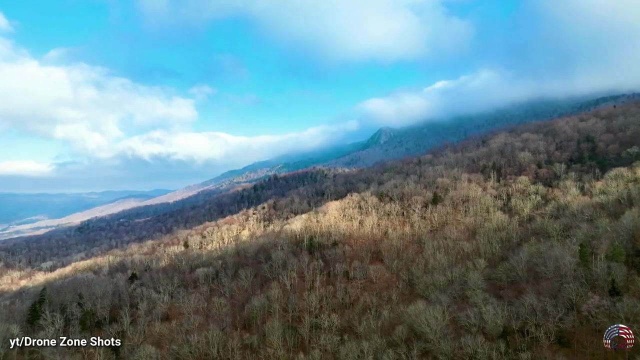 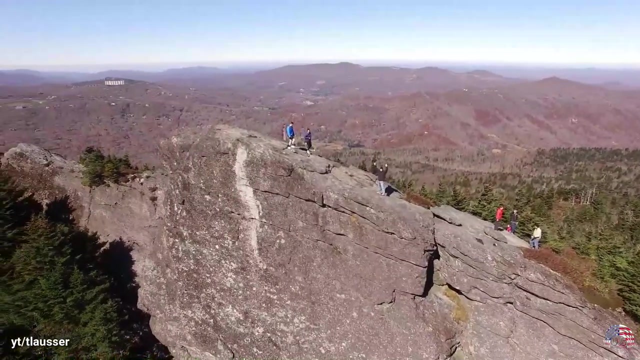 waterfalls. Grandfather Mountain. The mountain is a non-profit attraction located near Linville in North Carolina. It is 5,946 feet high and one of the most prominent chains in the Appalachian Mountains. Hiking on Grandfather Mountain ranges from easy trails with beautiful views to rugged hikes. 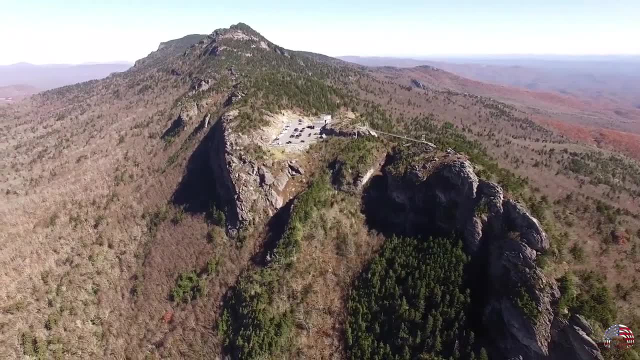 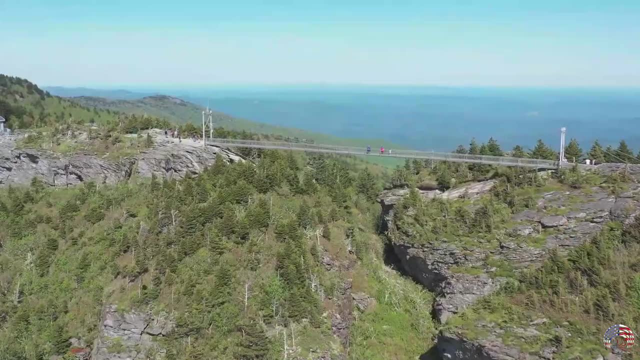 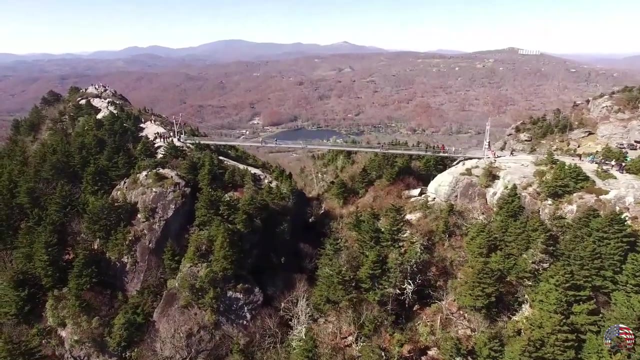 including ladders and rewards. with vast panoramic views, Visitors can also learn about the native flora and fauna or get a glimpse of wildlife. You can take a stroll along the park's famed mile-high swinging bridge, used since 1952, but now an attraction and provides 360 views. The mountain is also within easy driving reach. 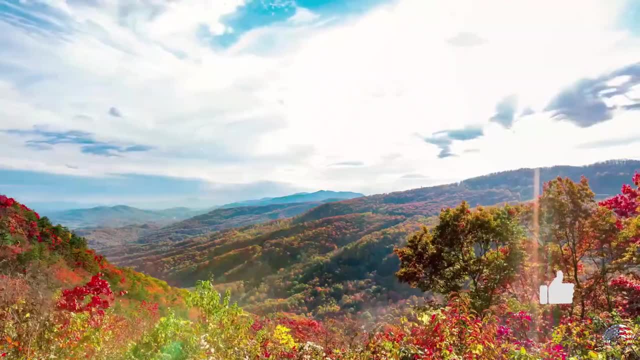 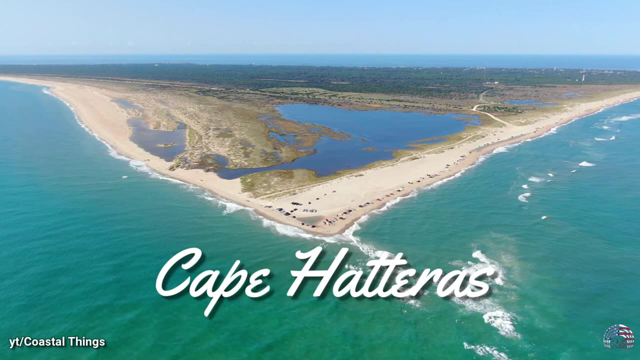 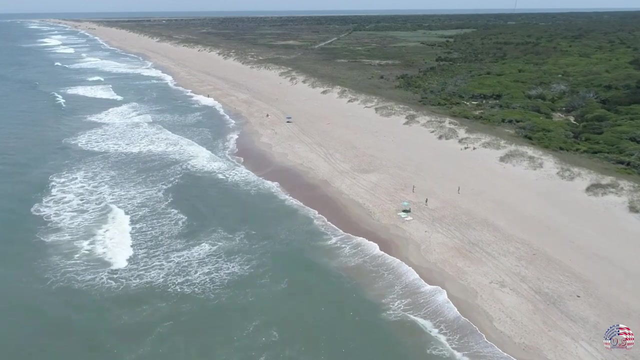 to the cities like Banner Elk and Blowing Rock. Cape Hatteras In the Outer Banks region, Cape Hatteras National Seashore was the first national coastal preservation zone and the crucial barrier island along the coast. The visitors are not only there. 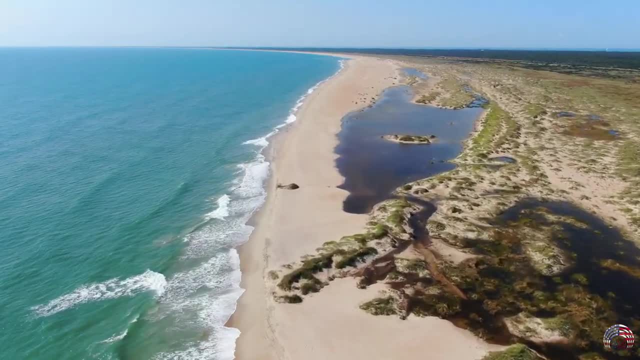 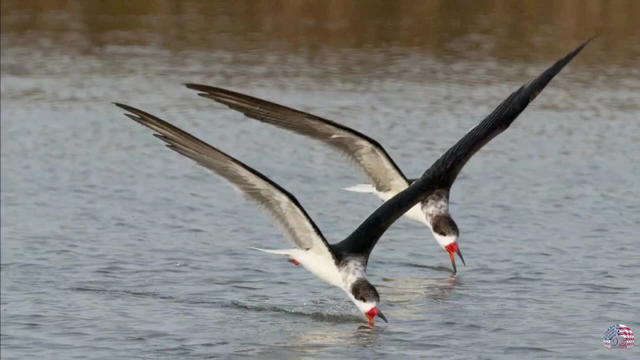 for the beaches. they also come for the distinctive biodiversity and the rich background. Bird watchers can look at the piping plevers, American Oyster Catcher, gull-billed tern and black skimmer. The beaches are home of several species of sea turtles. like an endangered, 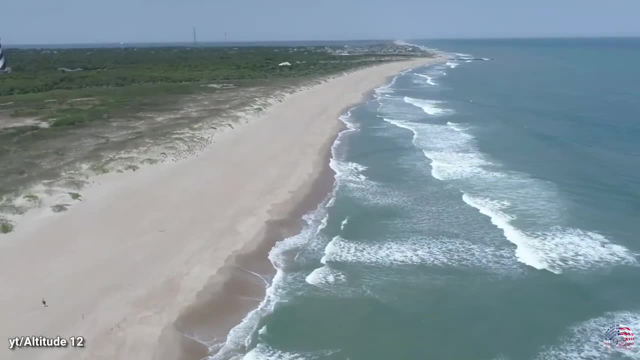 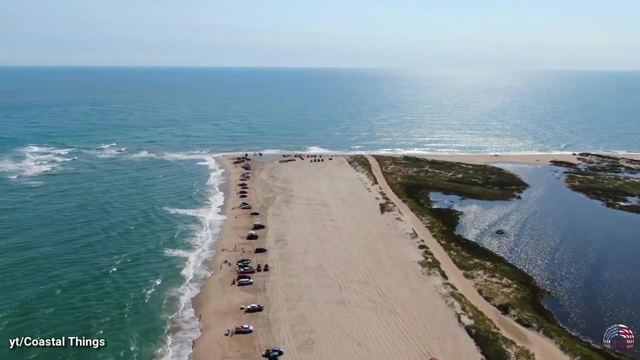 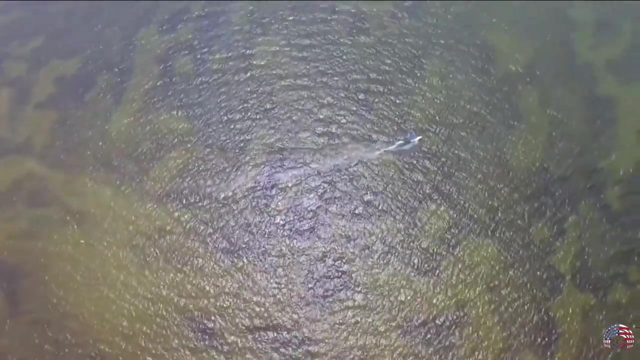 loggerhead sea turtle, and during winter you can spot seals lying on the beaches. Another popular thing is to visit Historic Lighthouse. Bodie Island Light Station is currently in its third edition, following the first one's instability, And the second one was destroyed during the Civil War. Cape Hatteras Light Station was originally constructed in 1803, and rebuilt in 1870.. It serves as a vital beacon in some of the more hazardous parts of the Atlantic Coast, where the Gulf Stream meets the Virginia Drift and is home to numerous shipwrecks. 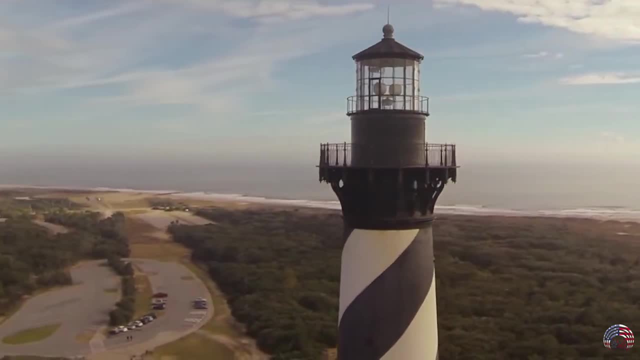 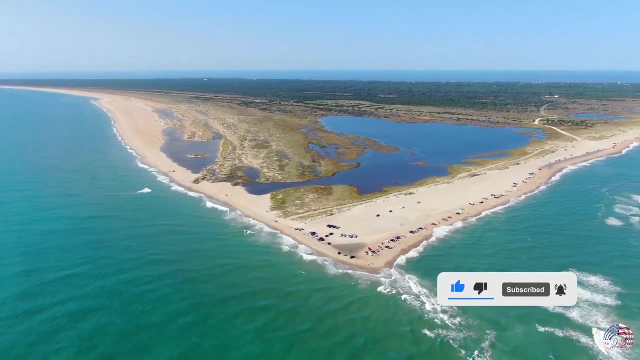 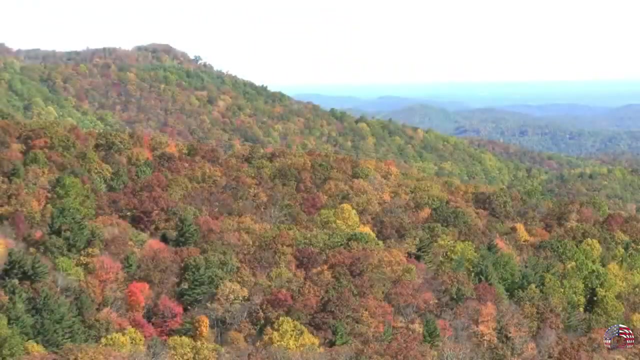 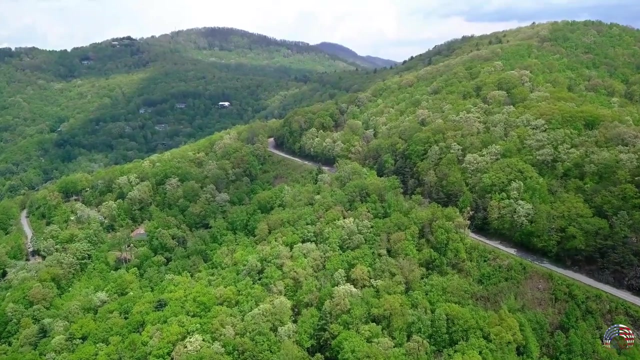 While it's not accessible to visitors, the Ocracoke Lighthouse has been operating since 1823 on the island Blue Ridge Parkway. It was dubbed America's favorite drive. the 469-mile parkway was designed by landscape architect Stanley Abbott. His vision was to create a road that was more than a means to connect. 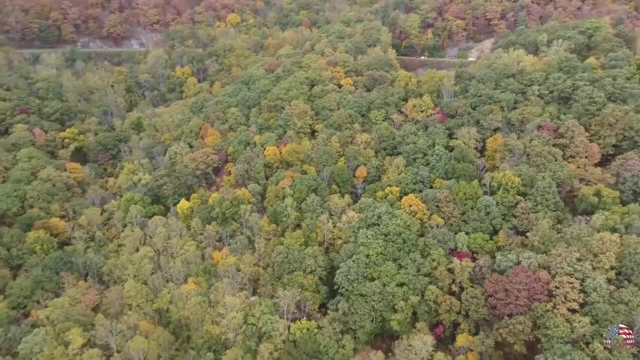 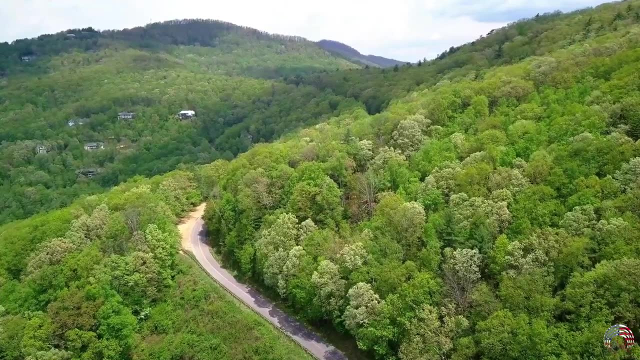 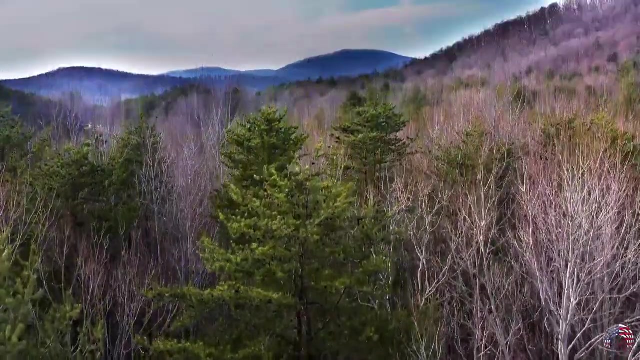 The Great Smoky Mountains National Park in North Carolina to the Shenandoah National Park in Virginia, The popular destination for bicyclists and motorcyclists for its breathtaking views. The drive is awe-inspiring, with beautiful views and panoramic views of Blue Ridge Mountains and the surrounding landscapes. 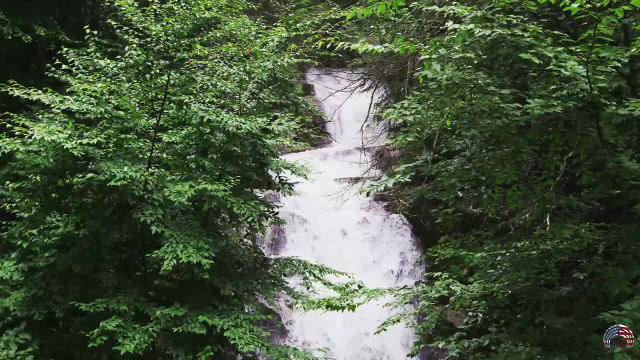 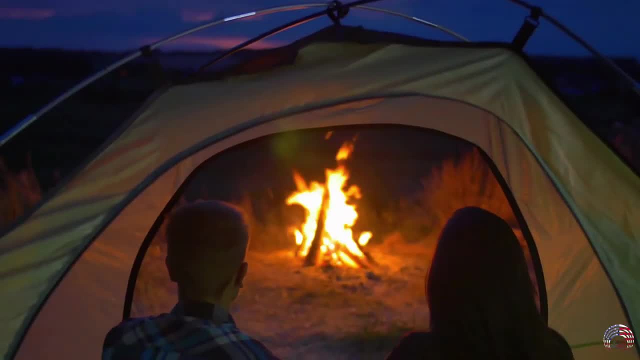 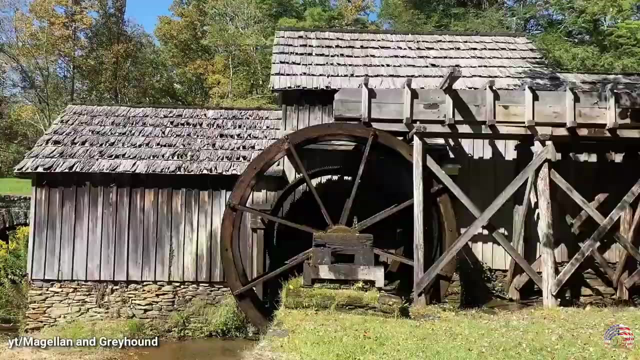 Along the way, you will find numerous hiking trails that lead to stunning waterfalls. Take a picnic lunch with you and then stop at the picnic spots. Are you a fan of camping? Many campgrounds are accessible all along the route. In the fall and summer, Mabry Mill offers demonstrations of crushing corn with the old mills. 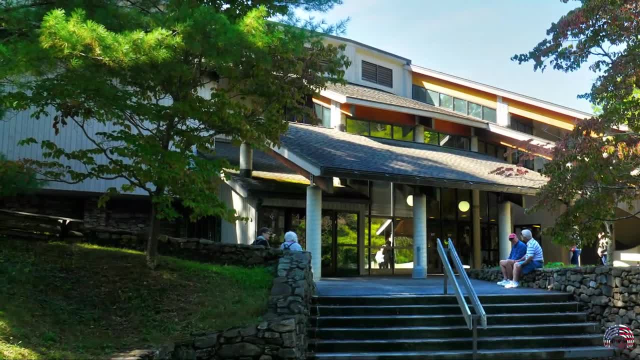 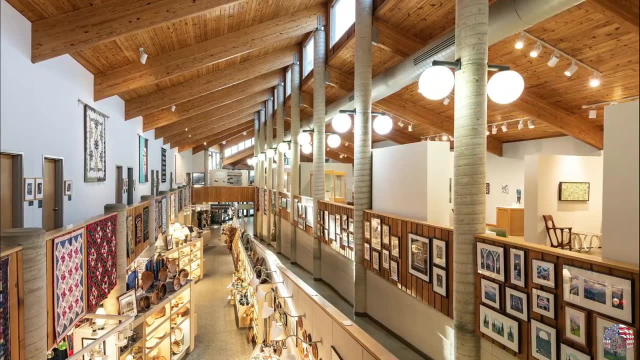 cutting boards inside the sawmill and blacksmithing. Folk Art Center is open throughout the year and is open to visitors every year and features a gallery of folk art, also demonstrations from local craftspeople. The parkway is more crowded during October's fall color, while summer visitors can enjoy. 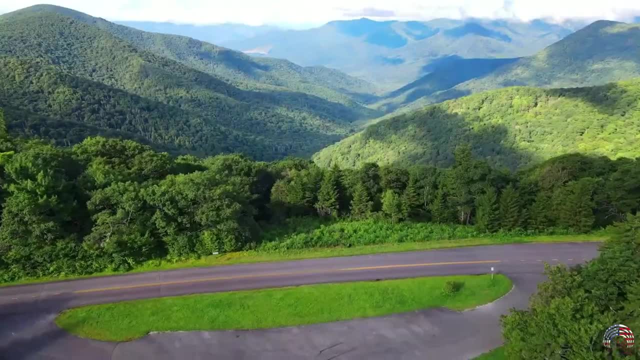 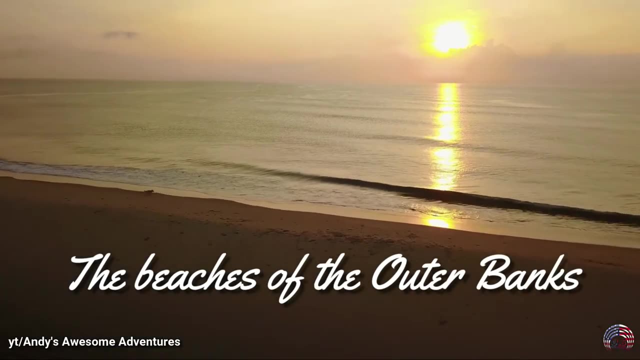 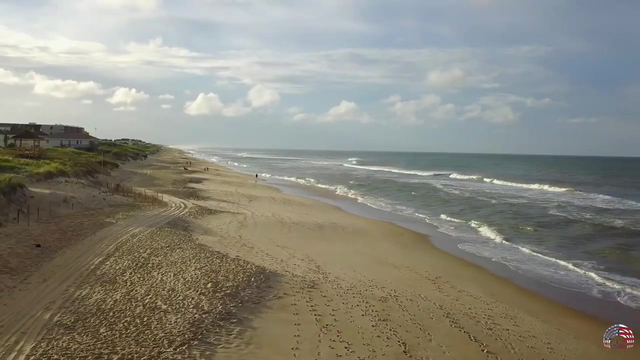 the vibrant colors of the flaming azaleas and rhododendrons, The Beaches of the Outer Banks. The Outer Banks, or it's called OBX by locals, a group of islands in the Barrier Reef area, is one of the most popular beaches in the Bay Area. 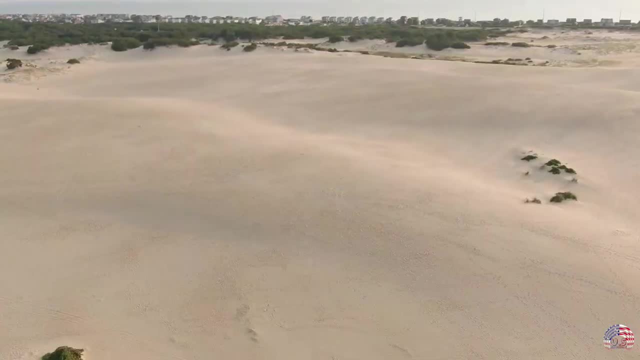 The Outer Banks, or it's called OBX by locals, is a group of islands in the Barrier Reef area, has auff silhouette and a southern view. Some ramen shops are open trong their years. There is also a return zone which includes Barrier凍, which es Phillip, Elway and the 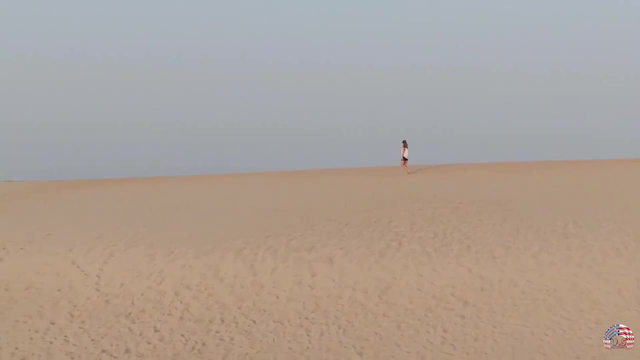 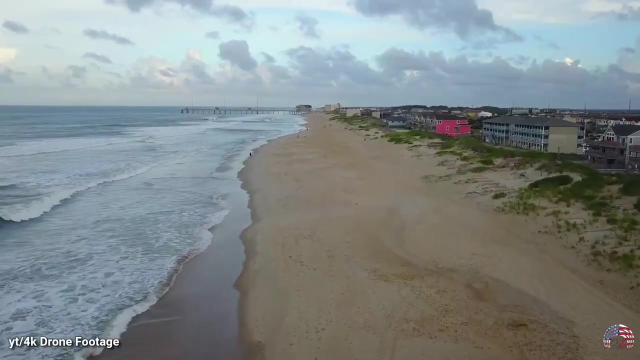 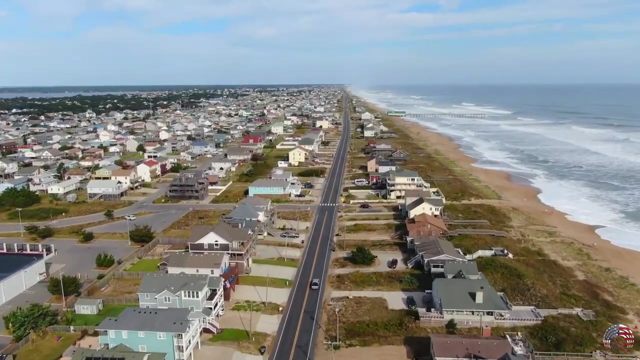 exciting Appellate House. It's a popular getaway for families who want to escape the summer heat. The hundred mile stretch of barrier islands is famous for its beautiful beach. Soft sand stretches along the coastline, drawing many visitors during the summer time. The Beachtowns of Nags Head, Kitty Hawk and Avon are the most popular destinations. 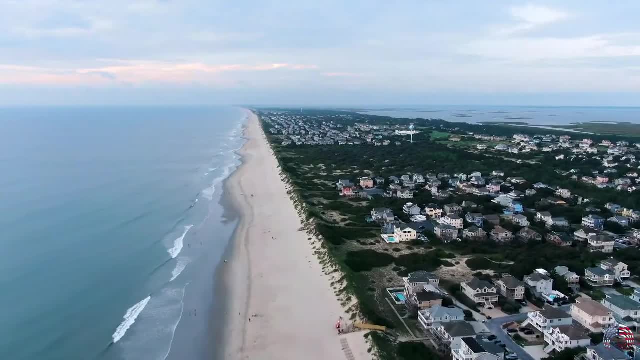 The big tiles in the beach卡LAarea of Las Vegas were bigger to explore. in those areas, The town of Nags Head offer a better variety of hotels and resorts than other towns. However, many individuals don't live on the beach floor. when traveling Sh전에는, Ohal or Menulineijnepad. 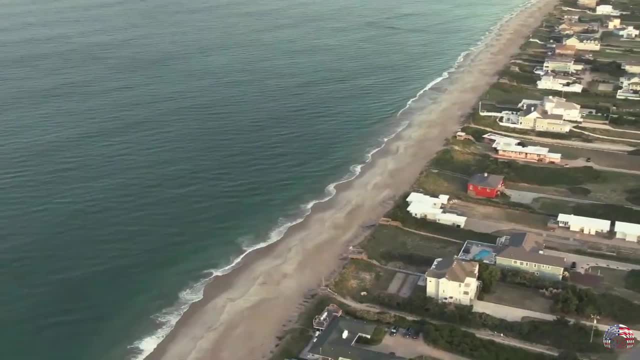 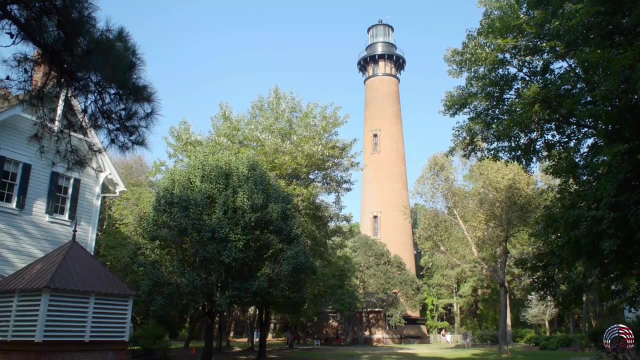 Gelda Yedil. Each town can XV Verizon aún più con el hotel Consular попадarte Con phosphorus. However, many individuals prefer to rent a cottage or beach house to enjoy the beach. Explore the area by visiting the History Center, lighthouses, spend a day and take a tour on. the Outer Banks Scenic Byway. Tourists visiting Roanoke Island can discover more about the lost town. Other tourist attractions within the region are the Elizabethan Garden at Fort Raleigh National Historic Site and Frisco Native American Museum. The northern portion of the Outer Banks is famous for the wild horses that roam its sand. 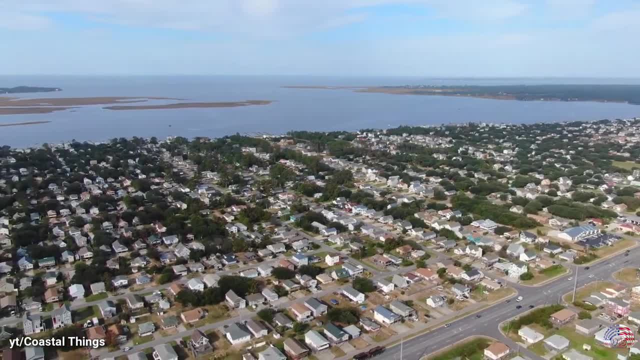 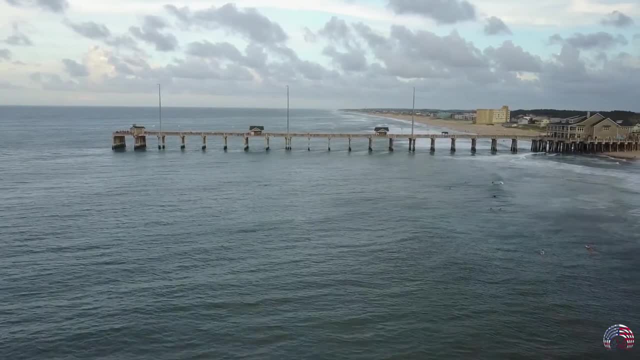 dunes. The middle part of the Outer Banks is the home of communities like Nags Head and Cutie Hawk. on Bodie Island, The town of Manio is the home of the lost colony, disappeared without a trace in 1580s. 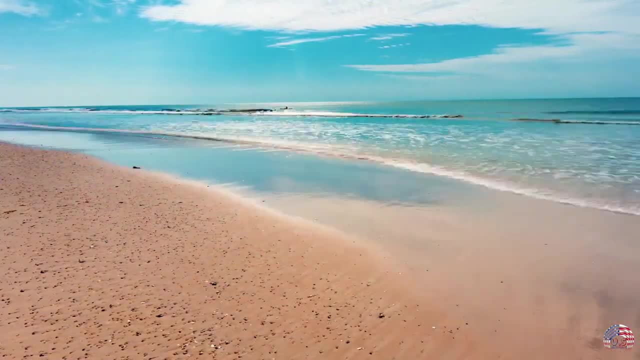 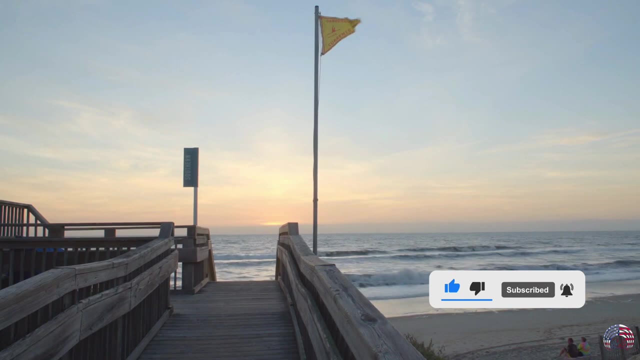 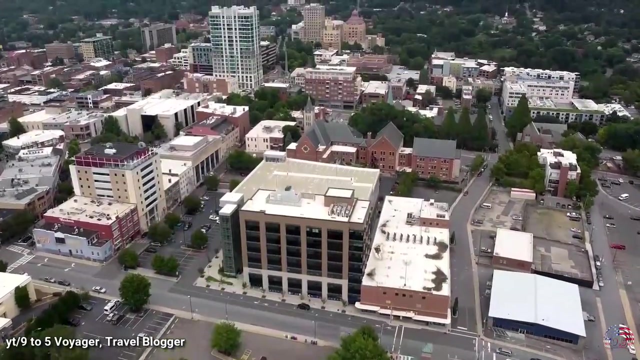 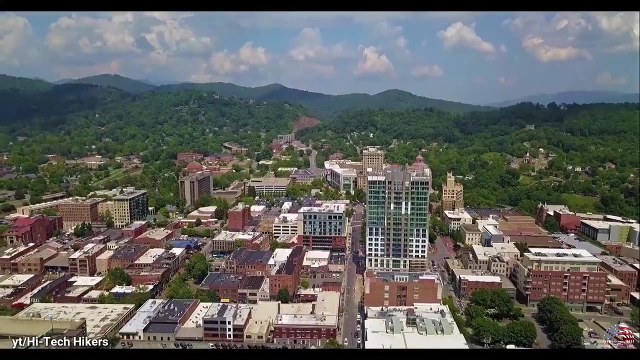 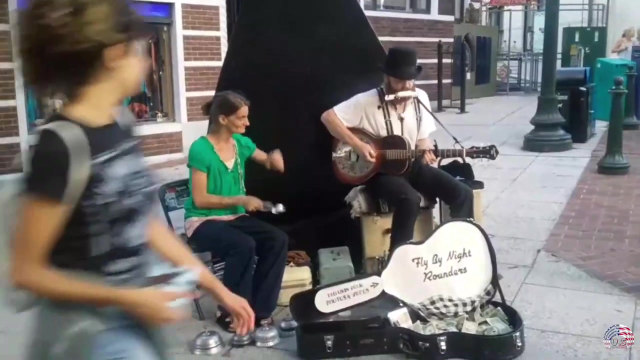 Further south is the gorgeous, quite natural Cape Hatteras Seashore and Cape Lookout National Seashore. The town is located in the stunning Blue Ridge Foothills and enjoys the reputation of being an active artistic community. The central area is home to several boutiques displaying local art, bars and fantastic restaurants. 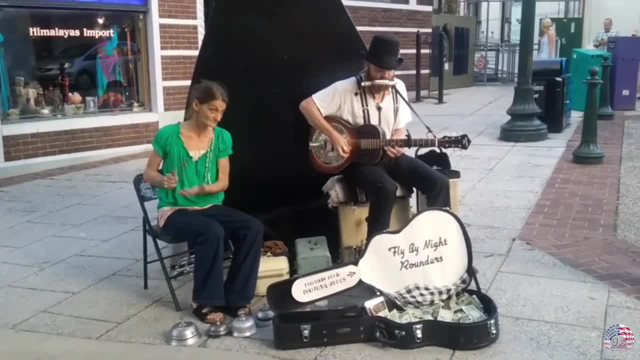 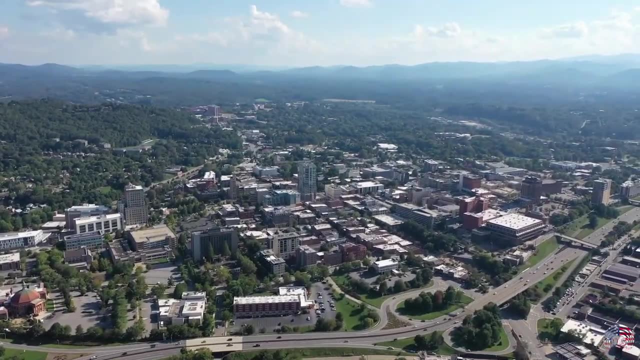 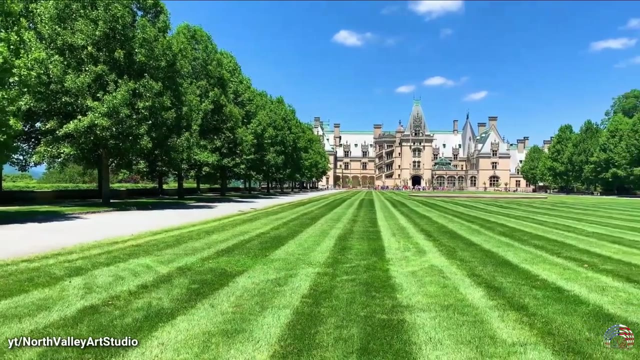 Street performers and musicians strolling through the streets enhance the overall artistic vibe. This charming and unique town has received numerous prizes and awards through many years, including America's Quirkiest Town, from Travel and Leisure in 2014.. Asheville is also close to the famous Biltmore Estate, built between 1889 to 1895. 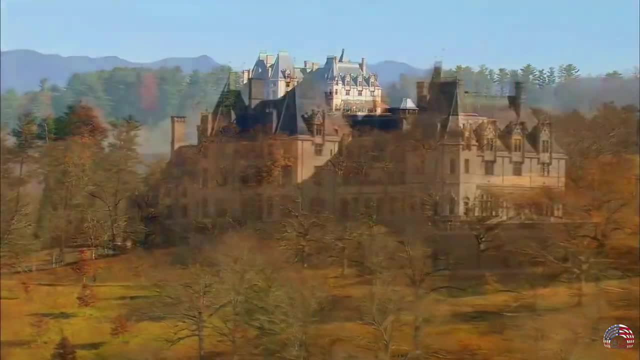 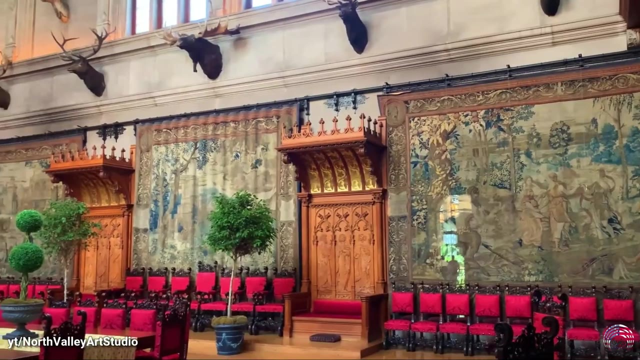 This chateau-style mansion is the largest privately owned house in the United States, covering 8,000 acres and attracting almost one million visitors every year. The estate is home to 250 rooms filled with unique paintings, antiques, architectural designs, collections of clothes and other accessories. 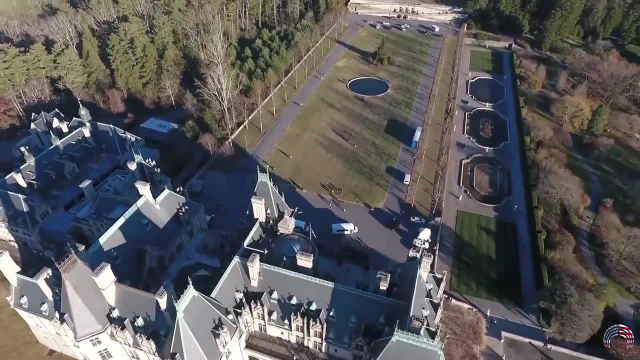 The estate is home to over 250 rooms filled with unique paintings, antiques, architectural designs, collections of clothes and other accessories. The estate is home to over 250 rooms filled with unique paintings, antiques, architectural designs, collections of clothes and other accessories. 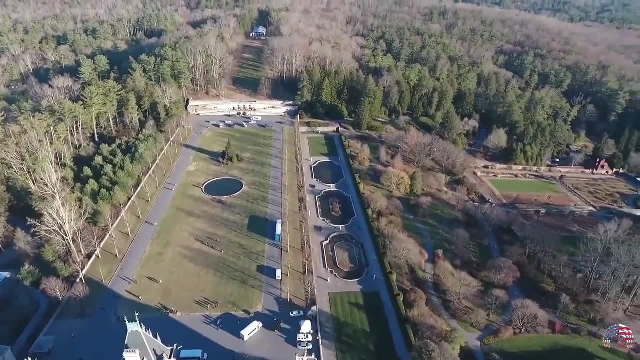 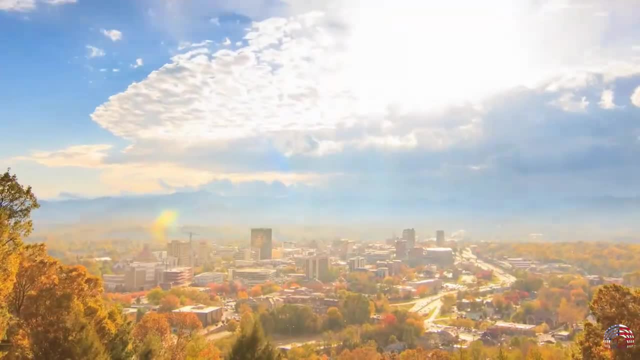 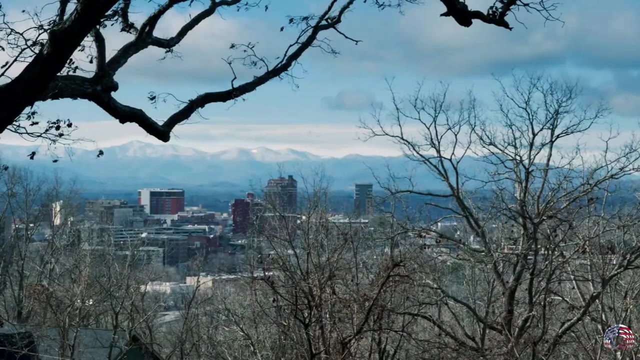 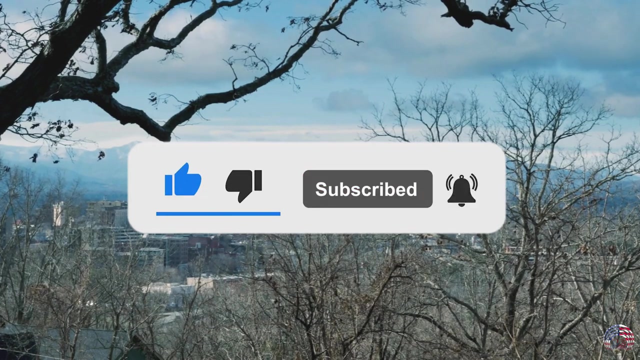 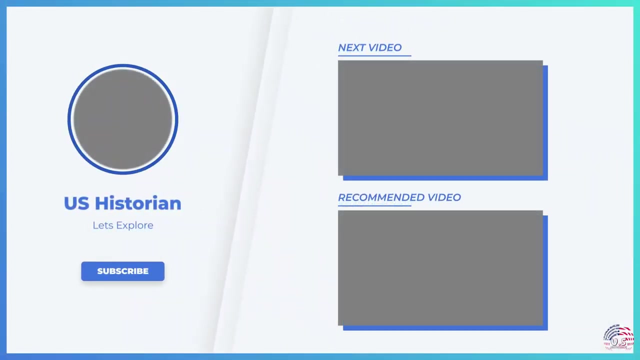 The several gardens are vast, with the Italian Rose Garden, intricate pools and sculptures. There are numerous dining options, entertainment and shopping. at Antler Hill Village There are numerousças of all interesting things that are owned, but their unique and unique style is one that is well-known in the community to which the town is one. The今年 ̶Lake Moodle, differential views and the~~.